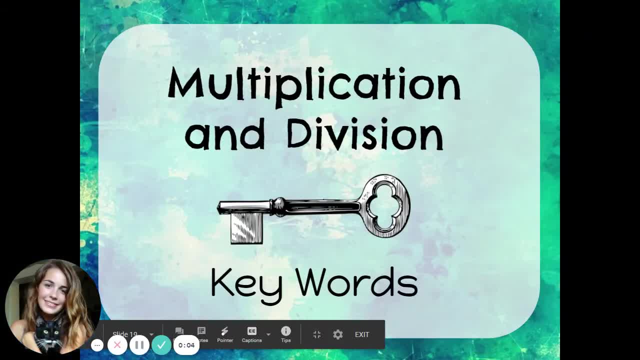 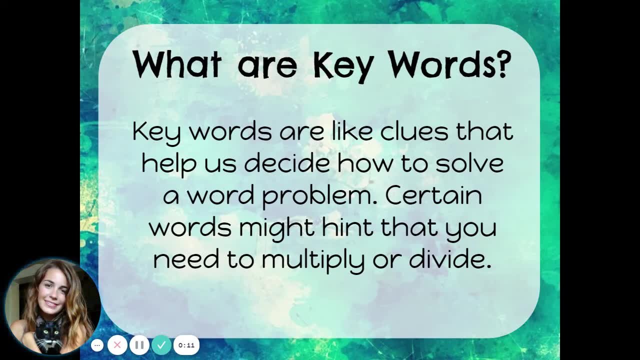 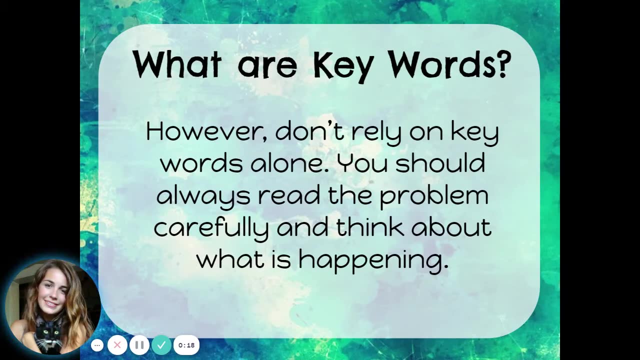 Multiplication and division keywords. What are keywords? Keywords are like clues that help us decide how to solve a word problem. Certain words might hint that you need to multiply or divide. However, don't rely on keywords alone. You should always read the problem carefully and think about. 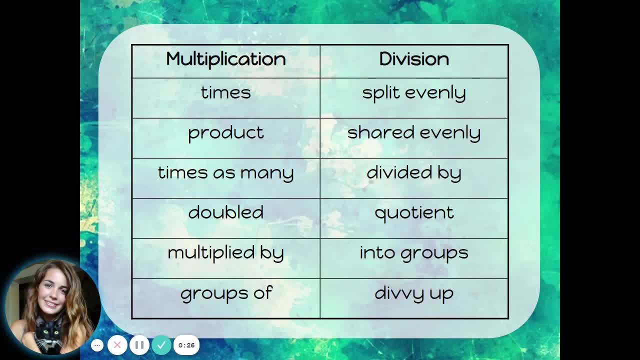 what is happening. Here are some words that might suggest you need to multiply or divide. Multiplication keywords include times, product times, as many doubled multiplied by, and groups of, While division words include split, evenly shared, evenly divided by quotient into groups. 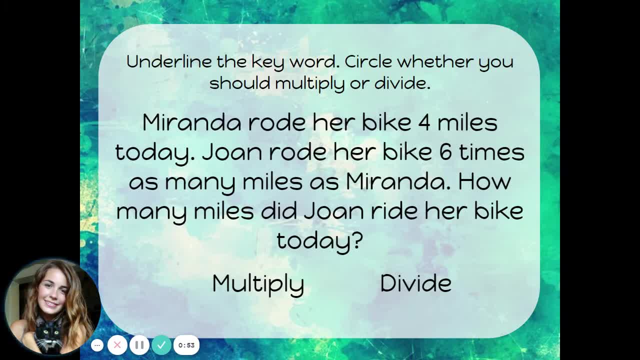 and divvy up. For each of these word problems, let's try to find the keywords and decide whether we should multiply or divide. Multiplication keywords include times, product times, as many doubled, multiplied by or divided. This one says Miranda rode her bike. 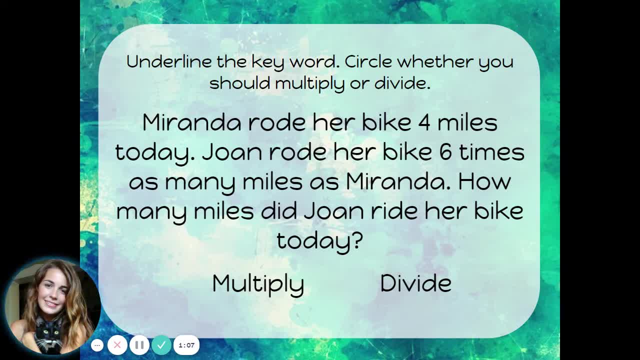 four miles. today, Joan rode her bike six times as many miles as Miranda. How many miles did Joan ride her bike today? Well, I see the words times as many and those are multiplication keywords. To solve this problem and figure out how many miles Joan rode, I would do four times six. 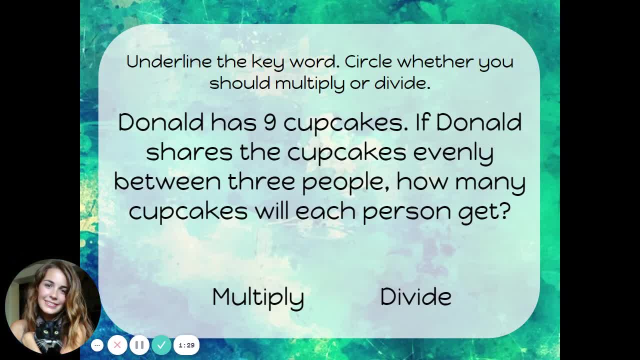 There's another. Donald had six are and had three, and not only. If he wanted to find the words. Donald has nine cupcakes. If Donald shares the cupcakes evenly between three people, how many cupcakes will each person get? This time, I see, shares evenly. 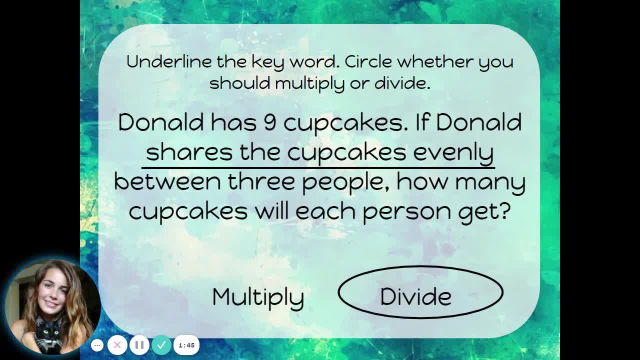 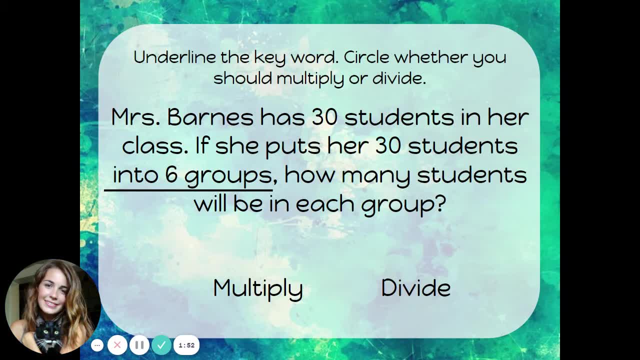 and if someone is sharing something evenly, that's division. Mrs Barnes has 30 students in her class. If she puts her 30 students into six groups, how many students will be in each group? This time, I see, into groups. We are dividing up 30 students into six groups. 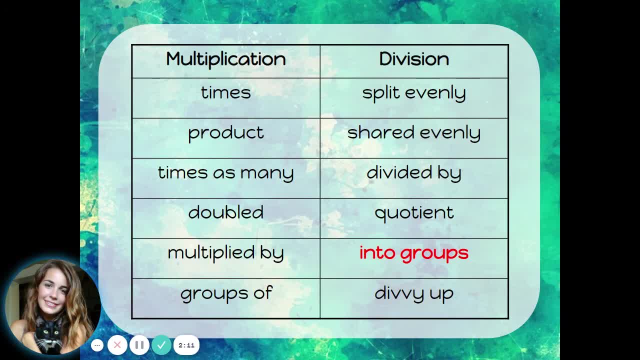 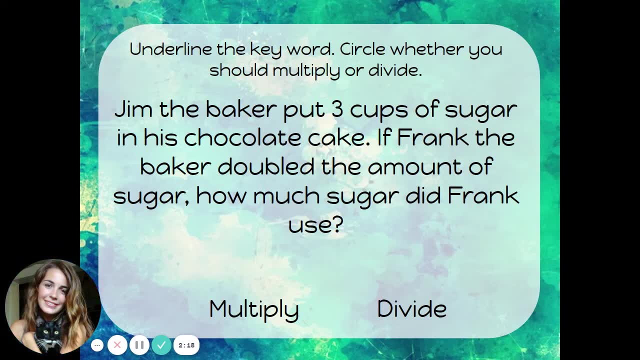 into groups. If you're putting something into groups, you're dividing. Jim the baker put three cups of sugar in his chocolate cake. If Frank the baker doubled the amount of sugar, how much sugar did Frank use? If you're doubling something, you're going to know this. We're going to divide nine into six groups.